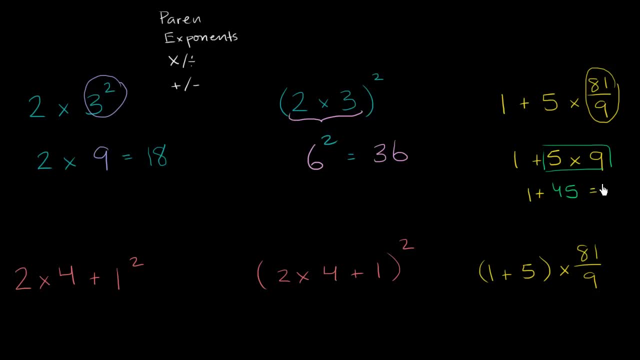 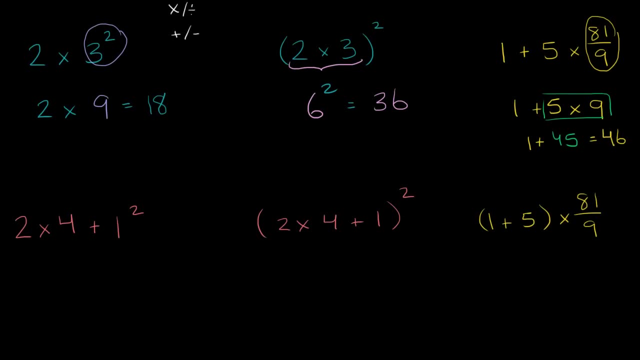 So this becomes 1 plus 45, which of course is 6.. Of course is equal to 46.. Now let's tackle this one right over here. So we would want to do the exponents first. So 1 squared, well, that's just going to be equal to 1.. 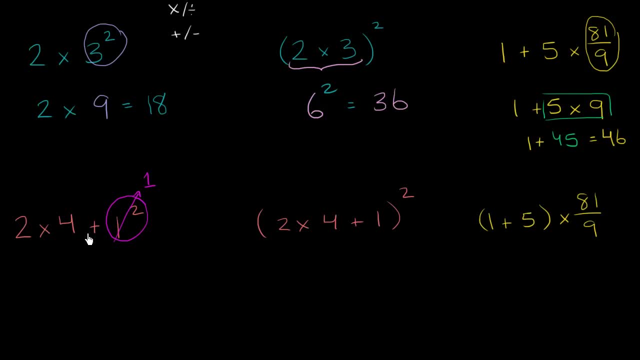 So that's just going to be equal to 1.. And so you have 2 times 4 plus 1.. What should you do? Should you add first or do the multiplication first? Well, multiplication takes precedence over addition, So you're going to do the 2 times. 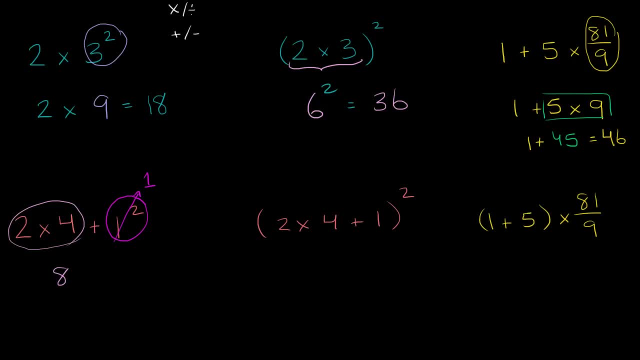 4 first. 2 times 4 is 8.. So you're going to have 8 plus 1, which, of course, is equal to 9.. Now you have a very similar expression but you have parentheses, So that's going to force you to do what's in the parentheses. 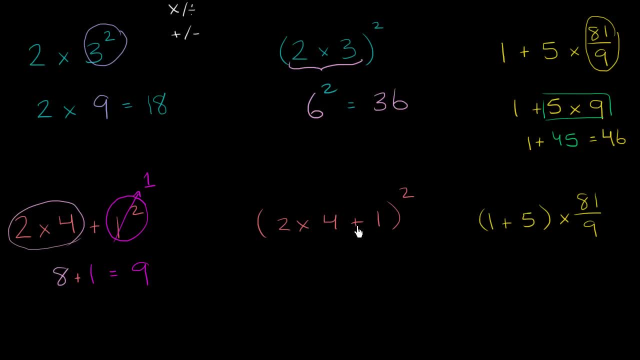 before you take the exponent. But within the parentheses we have multiplication and addition And we have to remember that we do the multiplication first. So we're going to do the 2 times 4 first. So that's going to be 8 plus 1.. 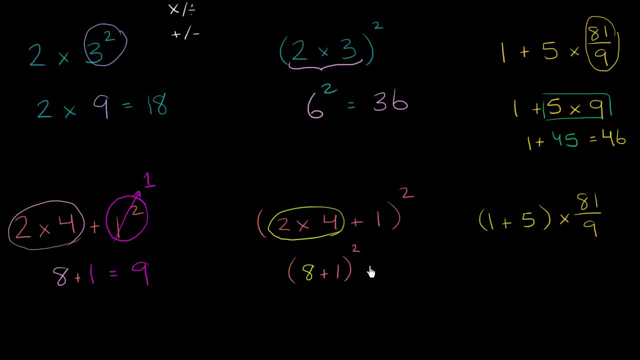 Plus 1 to the second power, 8 plus 1 is 9.. So that's 9 to the second power. 9 squared is the same thing as 9 times 9, which is equal to 81.. Now we have one more right over here. 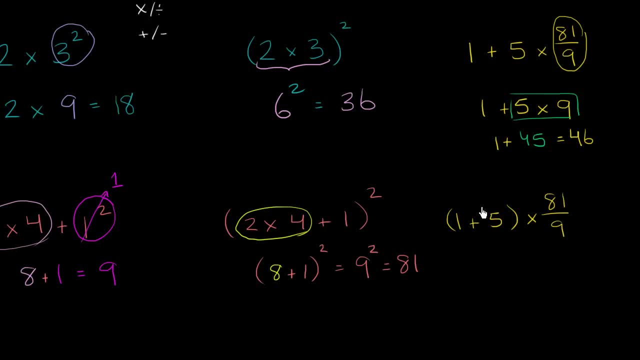 that looked very similar to this one, except once again we have parentheses. That's making us do the addition first. Without parentheses we would do the multiplication and the division first. But here we see that 1 plus 5 is 6.. 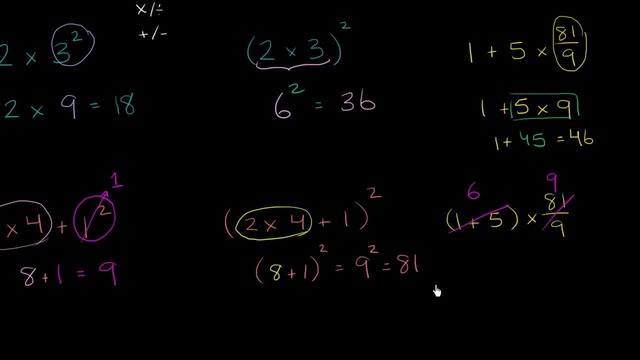 And then we have this 81 over 9,, which is 9.. So this simplifies to 6 times 9,, which of course is equal to 54.. 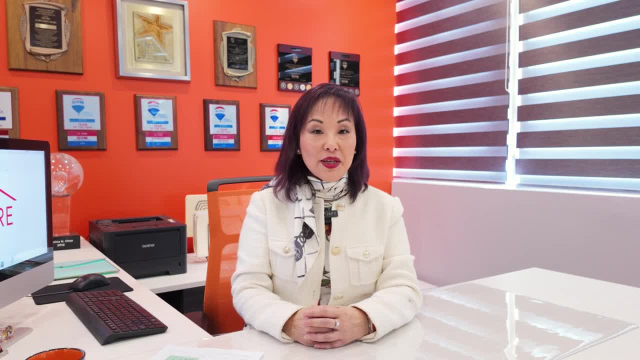 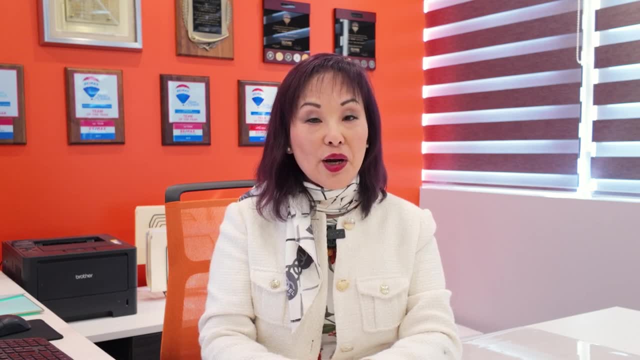 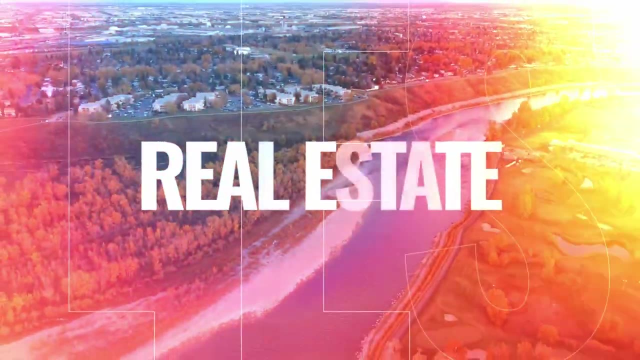 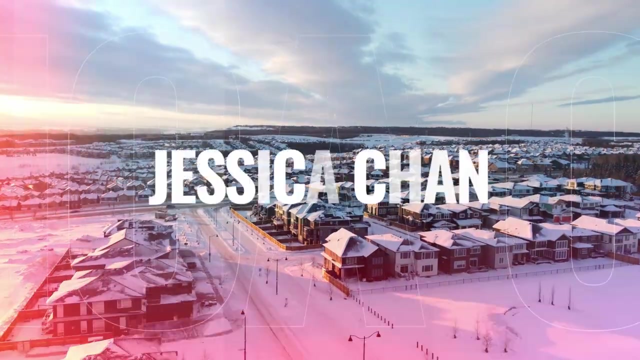 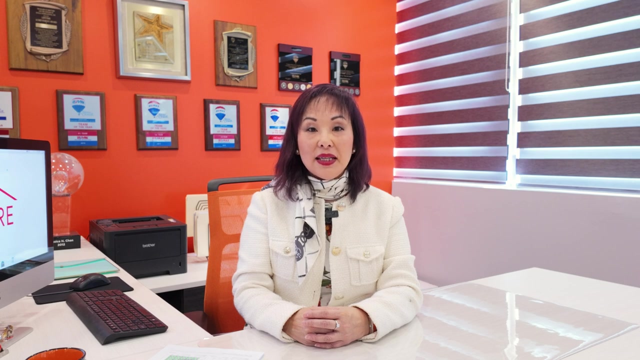 Are we still in a seller's market? How's the listing inventory in Calgary these days? Today, I'm going to share some valuable information that might interest you regarding Calgary real estate. This is Jessica Chan of JCRE and Management. March was another crazy month, as 1,151 single.